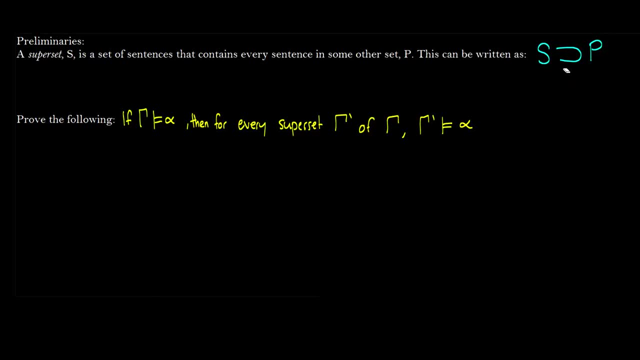 Sometimes there's a line under it, sometimes there's not. I'm not going to write it, but what this says in the Venn diagram, if you have. if all these sentences in this circle are P, then all the sentences will also be in some other set. 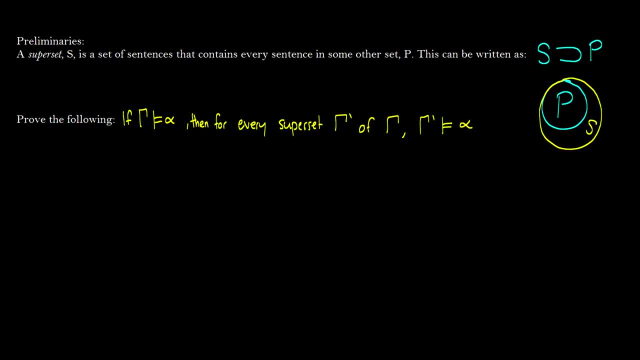 S. They're just going to be contained within, And there are some cases where S could possibly be the same size as P. technically a superset. Yeah, it is a superset. It's not a proper superset, but it's a superset. 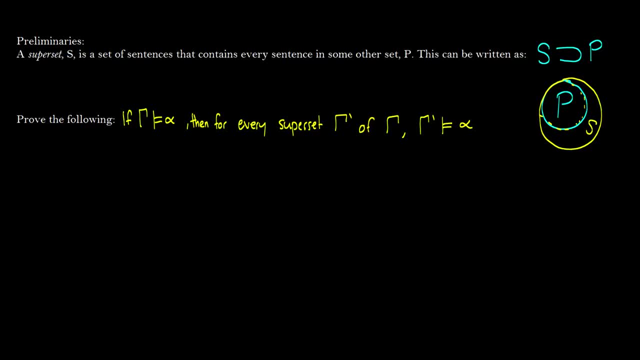 So using this, we are going to prove the following: If gamma entails alpha, then for every superset, gamma prime of gamma, gamma prime is also going to entail alpha. So this might seem a little daunting, because this is the first time I'm really introducing a ton of Greek letters. 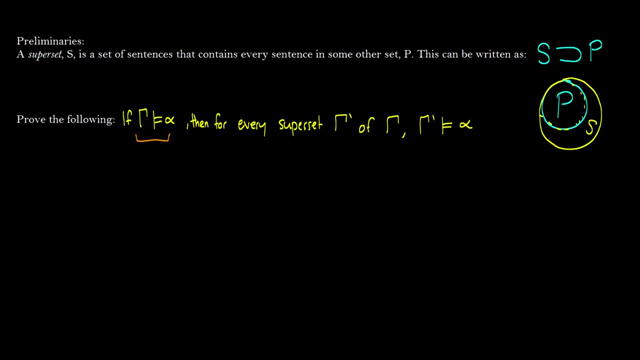 but basically what this says is that if we have a bunch of sentences P, Q, R, blah, blah, blah and we can get a truth-by-truth table of, say, some sentence S, then if we have another set that also contains 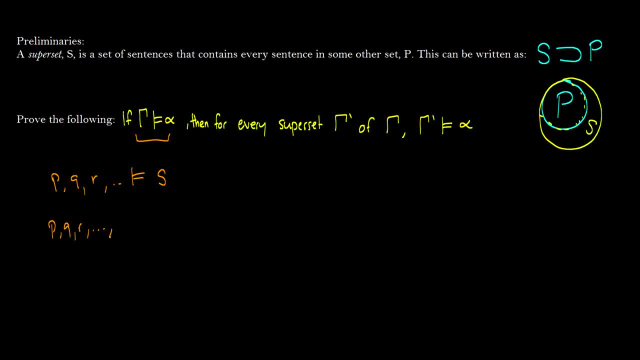 P, Q, R, blah, blah, blah. plus say: we have some other things in here- alpha, beta, gamma and some other things- then we can also get a proof of S from it. That's what we're saying. 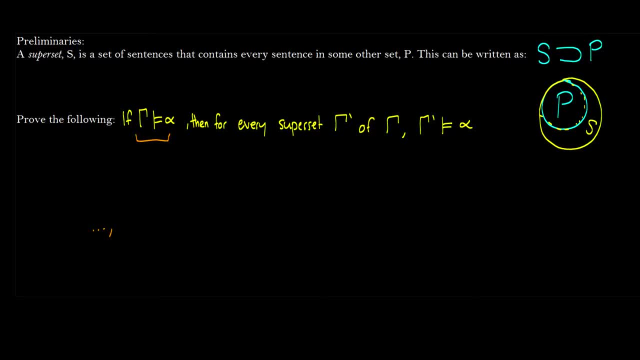 So what we're going to do is we're going to say: okay, well, we have our supposition that gamma proves alpha. So we say: gamma prime is a superset of gamma. therefore, every sentence in gamma, which this just means in: 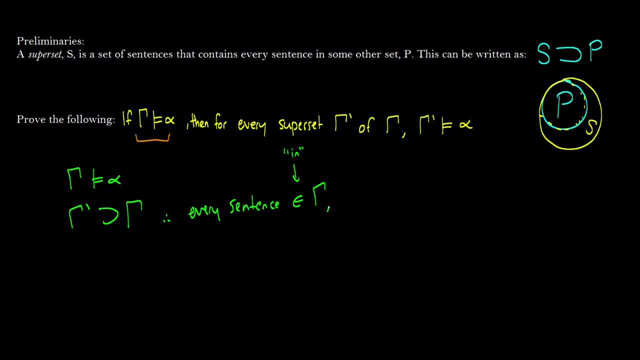 so every sentence in gamma is in gamma prime. Therefore, gamma prime will also entail alpha, because there is a proof um, because there is a proof of alpha in gamma. So because gamma prime contains gamma and alpha is proved in gamma, 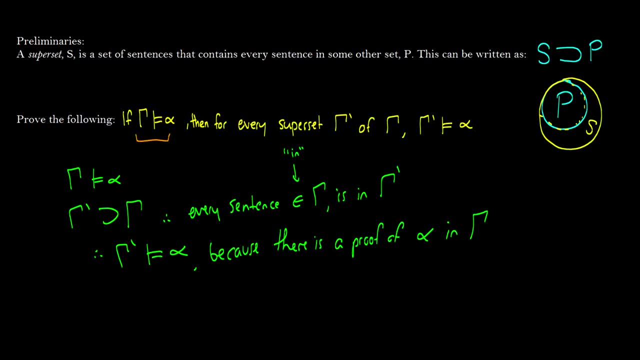 the bigger set also proves alpha. So entails is really the word I should be saying, but I think it's fairly intuitive. If we have this circle here, we'll call this gamma, and through this we get this lovely result of alpha. 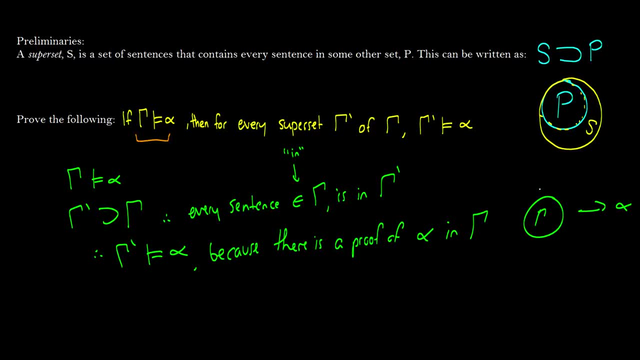 which please stop doing this. If we take a bigger subset of it- gamma prime- well, this area here is the one that proves alpha. So well, it's inside of gamma prime, therefore it also proves alpha, And I think pictorially is a great way to picture this. 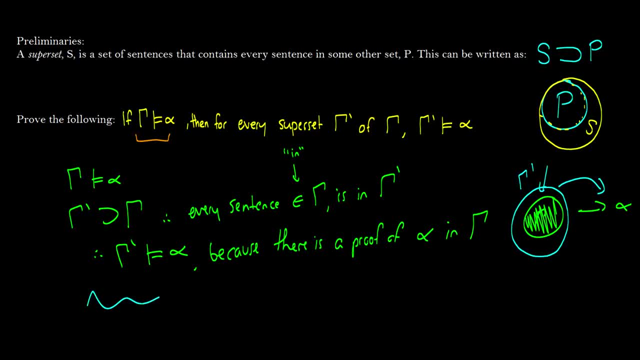 Obviously in a proof you wouldn't write that, You'd write down these lovely words. But hopefully as a first-year logic student, especially if you're just from philosophy and not doing math, it's not going to be as daunting to see a picture proof like this. 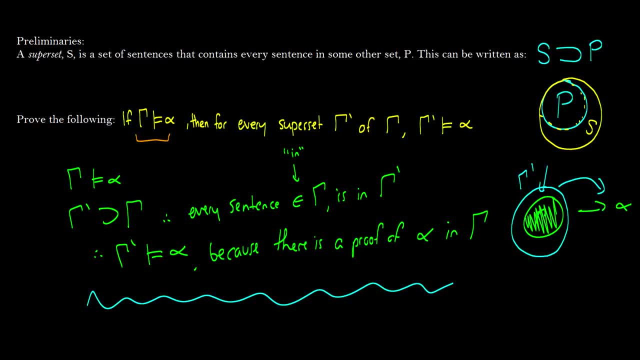 And you need, you need, need, need, need, need to get used to using these Greek letters and these sort of definitions. It's scary, but when you have the pictures and you know the notation, it's very easy to just put things together. 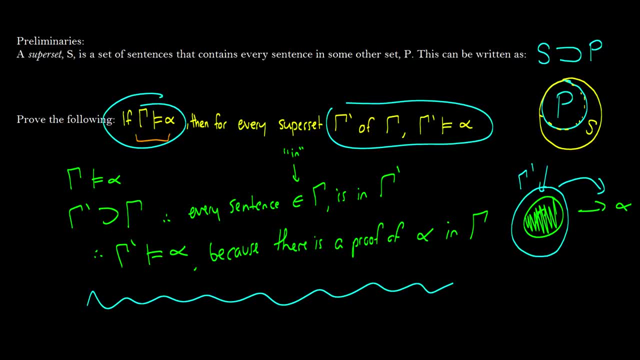 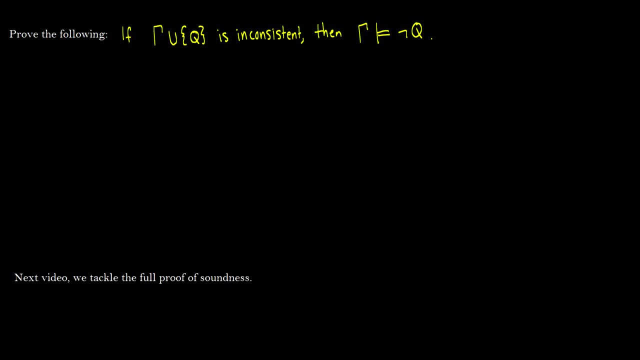 So there is one proof, And on this page there's another one we're going to prove, and that we have a new operator here. This is called the union operator, So this just kind of means like gamma and Q. 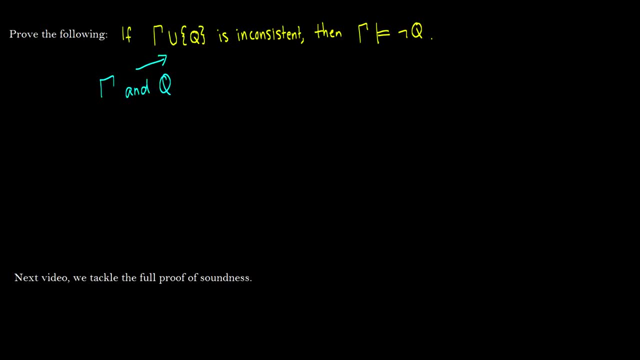 not in the sense of and as in truth tables, but it contains both gamma and Q. So this is what this means. So if gamma and this new atom Q is inconsistent, which means it's a contradiction, then gamma is going to entail the negation. 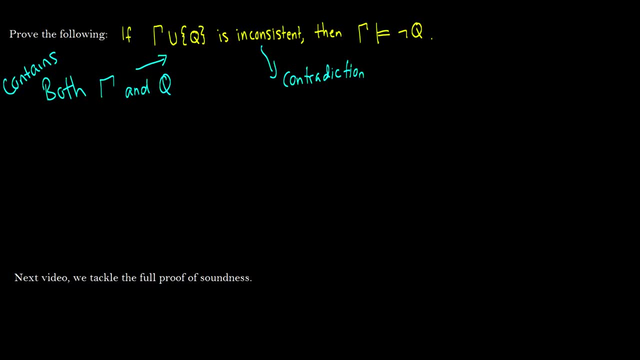 of that consistency. So here's what we'll do. We'll start this proof off nicely. Okay, So we're going to assume that gamma is consistent, meaning that there are no contradictions, And then we'll assume that gamma union Q. 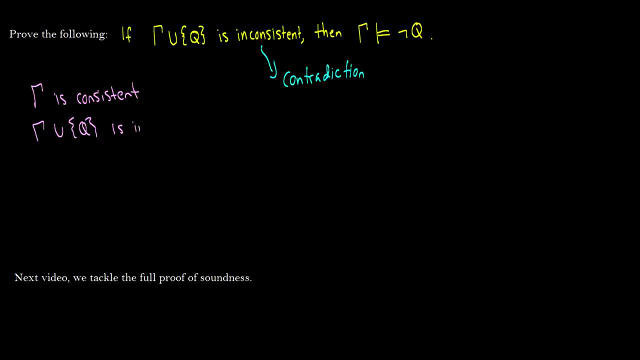 so when we take Q into it, it's going to be inconsistent. So therefore we have that gamma union. Q is going to prove some false theorem which we write like this: I'm actually going to leave this line out, because that's something a little bit. 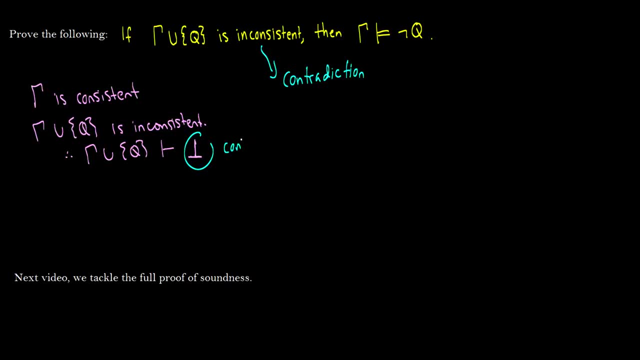 Actually, I'll just leave it here. This is the symbol for a contradiction. This is called the fulsome, and it just means there's a contradiction. So what it should be is an entailment symbol. What it should be is an entailment sign here. 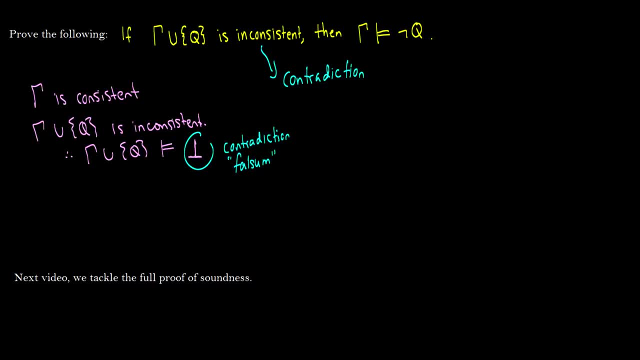 So gamma union, Q is going to entail the fulsome. Therefore, Q creates a contradiction, So Q creates a contradiction, And we know that any contradiction can never be true. Therefore, gamma is going to entail the negation of it. 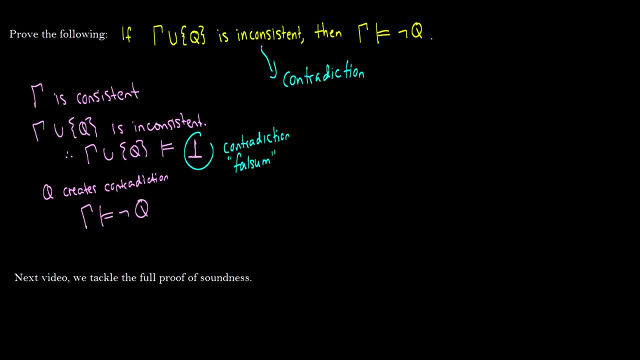 And the reason I say this is because, okay, if we have gamma union Q, let's just write this as gamma comma Q, and it proves some sort of inconsistency. then that means that inside gamma is a proof of not Q, And because there's a proof of not Q, 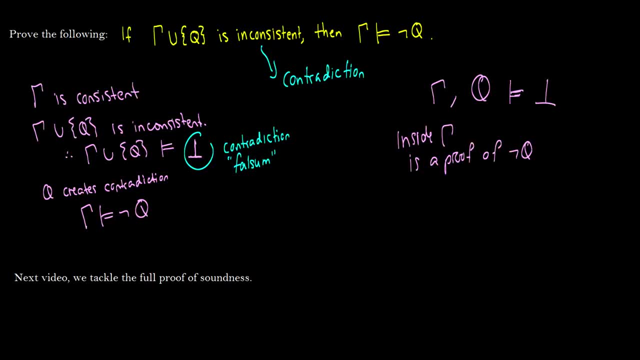 inside gamma. when we add Q to our system, it is going to create a contradiction. Therefore we cannot add Q. So that means that if we have gamma, we should be able just to prove, not Q on its own, Because adding Q makes a contradiction. 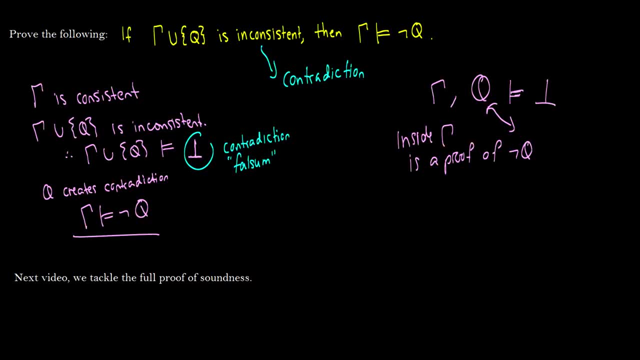 Therefore, not Q- must be inherently part of the system we already have, which is gamma, And I think that's probably one of the easiest ways to explain it. There are much more technical words in textbooks, but I'm trying to distill it down.